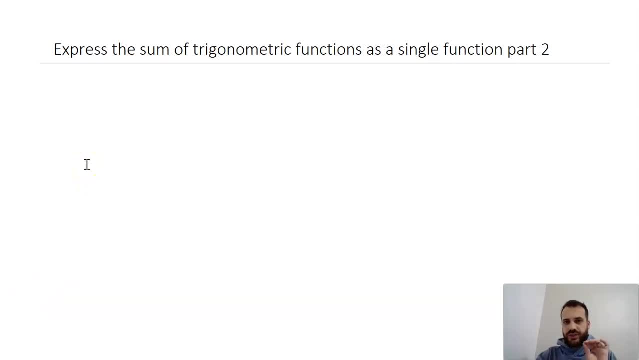 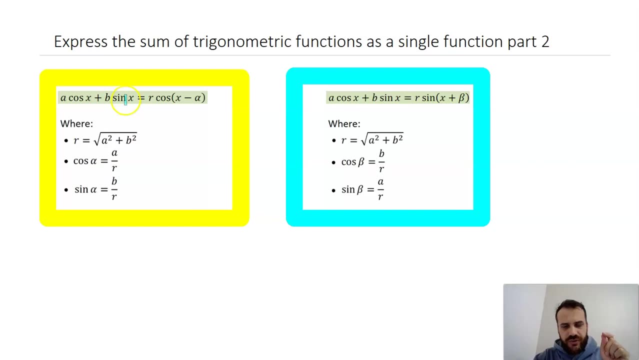 All right. so this is part two of express the sum of trigonometric functions as a single function. Now recapping, these are the things you need to know. So if you have a cosine function and a sine function, you can add them together to make a single cosine function where r is a squared plus. 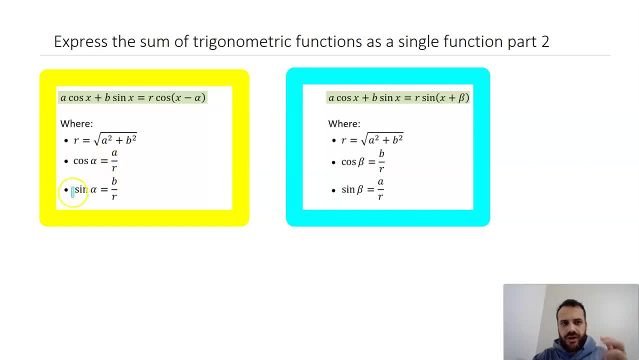 b squared and cos alpha is equal to a over r and sine alpha is equal to b over r. You can also add together the same functions- a cos x plus b sine x- and get r sine x plus beta instead, and where all of that is also true. Okay, so that's where we're at Now. if we were to go and do an example like: 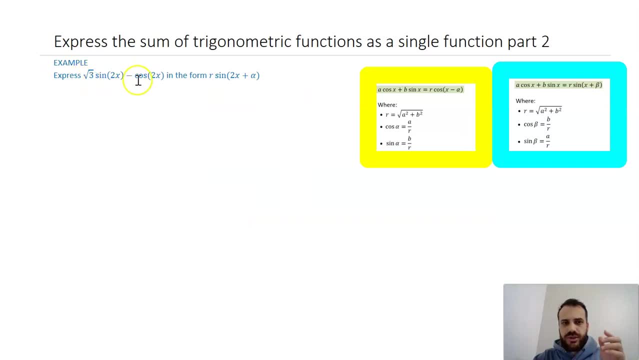 this express root 3 sine 2x minus cos 2x, in the form r sine 2x plus alpha. Now how are we going to use these formulas when these it's not x, it's 2x? Well, the easiest way to do it is to just let 2x equal some other letter and then proceed as. 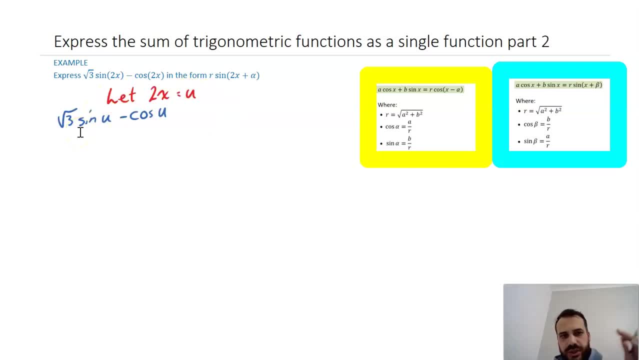 normal Let 2x equal u. the equation becomes much simpler: root 3 sine u minus cos u, and I can start working with that. Now I really need to know what that r value is. A value? here I take my b value. 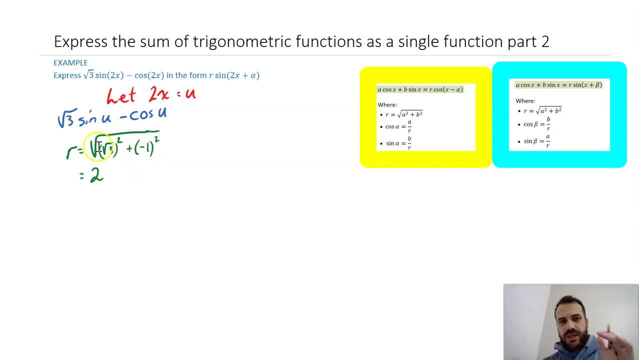 here, I add them together. sorry, I square them. I add them together, I square root them. I get an answer of 2, my r value is going to be 2. And my next job is to figure out what this alpha value. 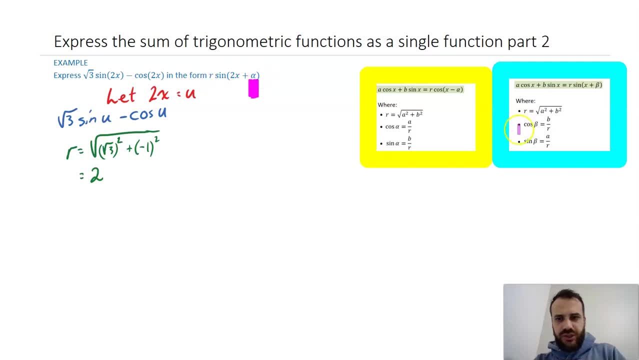 is here And because I'm trying to create a sine function, I'm following this information here. So it's going to be cos alpha equals b over r and sine alpha equals a over r. So I've subbed in my values here. Now you need to be really careful here, because my equation here is a cos x plus b. 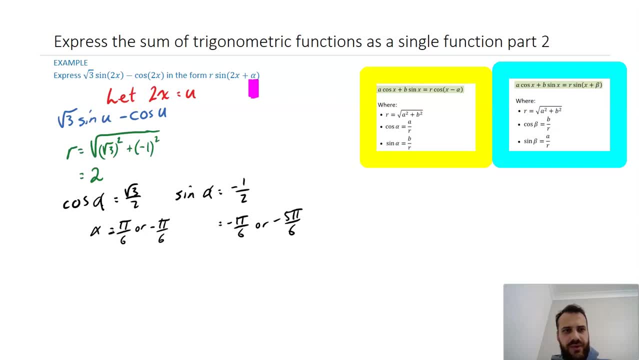 sine x. but this is written in the reverse, So our b value here is not negative 1, our b value here corresponds with our b value here, Root 3.. So that means that cos alpha is going to be root 3 over 2 and sine alpha is going to be 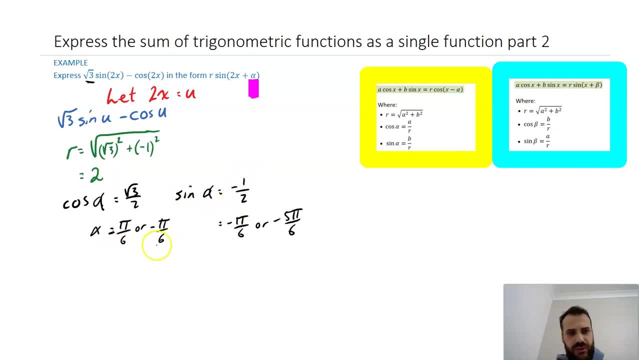 negative: 1 half. Now we're going to get two values when we solve here. It's positive here, so that's going to be in quadrant 1 or quadrant 4.. And this one's negative, so it's going to be in quadrant 4.